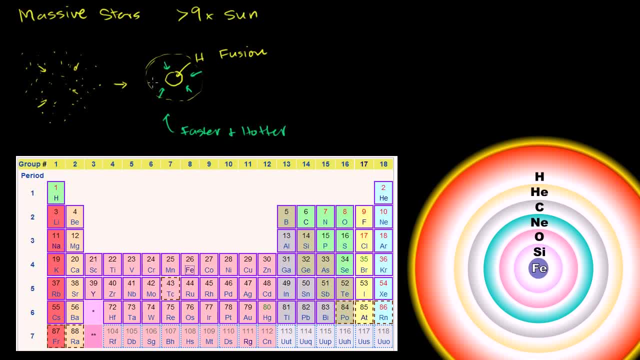 Faster and hotter, And so even this stage is going to happen over a much shorter period of time than for a star. the mass of our sun, Our sun's life, is going to be 10 or 11 billion. Here we're going to be talking about things in maybe the tens. 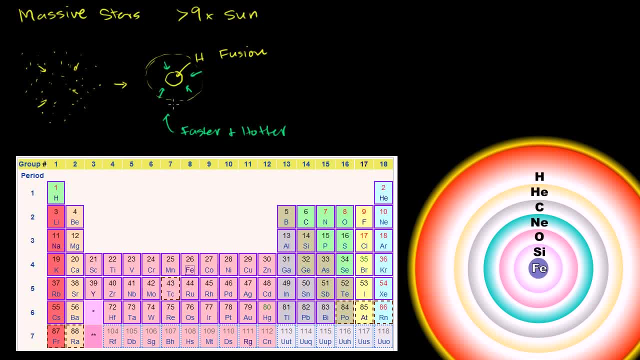 of millions of years, so a factor of 1,000 shorter lifespan. But anyway, let's think about what happens And so far just the pattern of what happens. it's going to happen faster because we have more pressure, more gravity, more temperature. 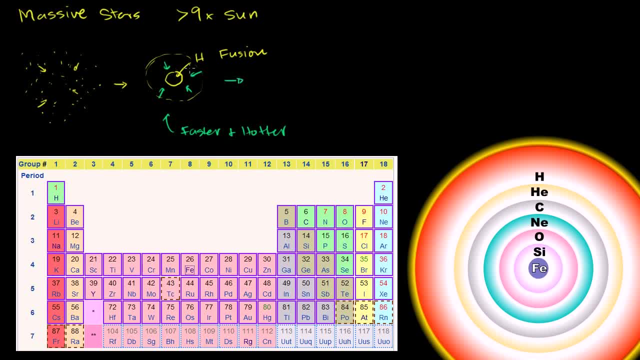 But it's going to happen in pretty much the same way as what we saw with a star: the mass of the sun. Eventually, that hydrogen is going to fuse into a helium core that's going to have a hydrogen shell around it. It's going to have a hydrogen fusion shell around it. 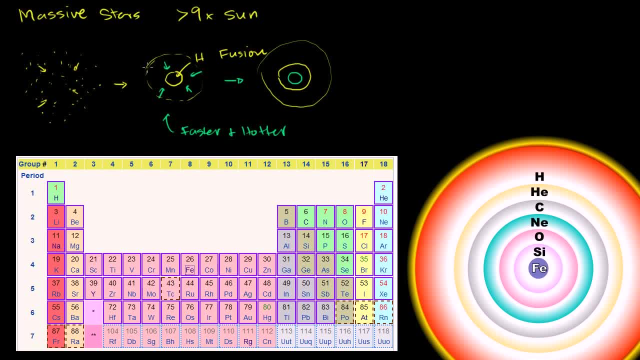 And then you have the rest of the star around that, So let me label it This: right here is our helium core, And more and more helium is going to be built up as this hydrogen and this shell fuses, And this is in a star the size of our sun. 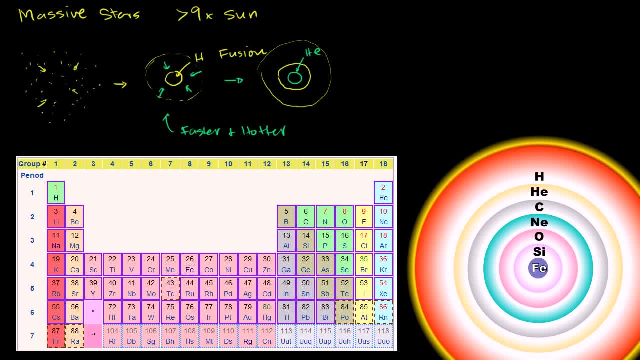 or the mass of our sun. this is when it starts to become a red giant, Because this core is getting denser and denser and denser as more and more helium is produced And as it gets denser and denser and denser. 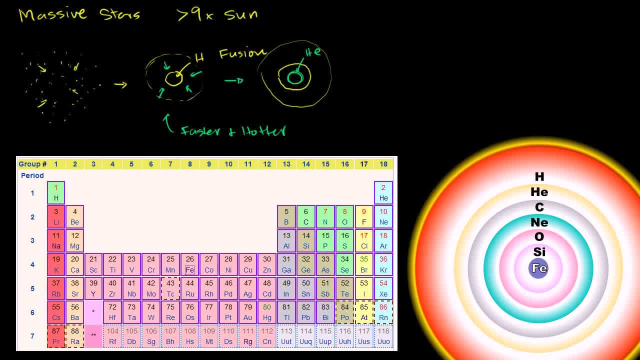 there's more and more gravitational pressure being put on this hydrogen shell out here where we have fusion still happening, And so that's going to release more outward energy to push out the radius of the actual star. But then when you fast forward there, so the general process. 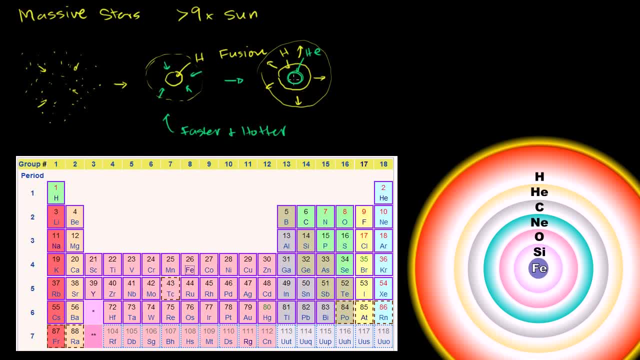 and we're going to see this as the star gets more and more massive is we're going to have heavier and heavier elements forming in the core. Those heavier and heavier elements, as the star gets denser and denser, will eventually ignite. 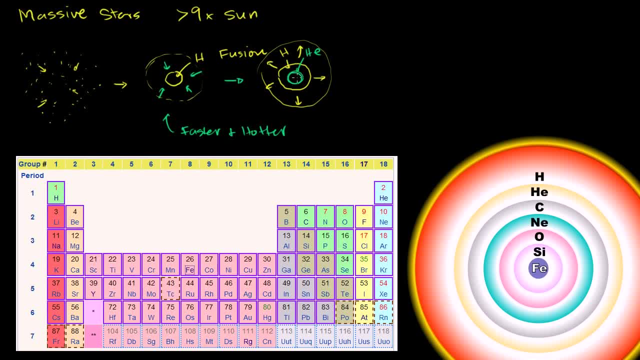 kind of supporting the core, But because the core itself is getting denser and denser and denser. material is getting pushed further and further out, or with more and more energy, Although if the star is massive enough, it's not going to be able to be pushed out. 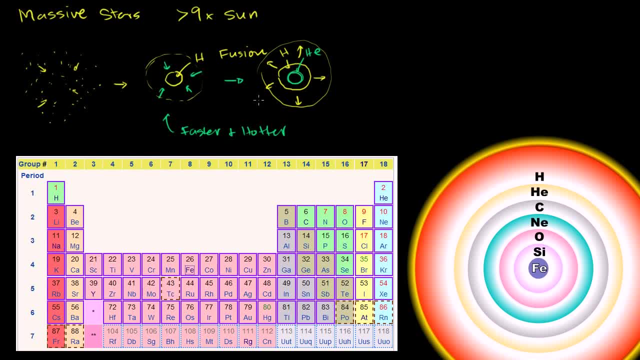 as far as you will have in a kind of a red giant with kind of a sun-like star. But let's just think about how this pattern is going to continue. So eventually that helium is going to, once it gets dense enough, it's going to ignite. 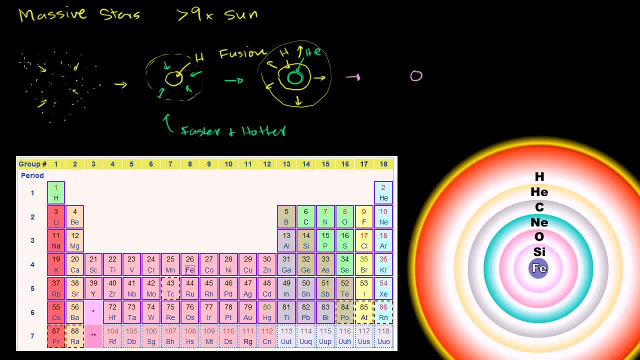 And it's going to fuse into carbon And you're going to have a carbon core forming. So that is carbon core, That's a carbon core. Around that you have a helium core. You have a helium core And near the center of the helium core, 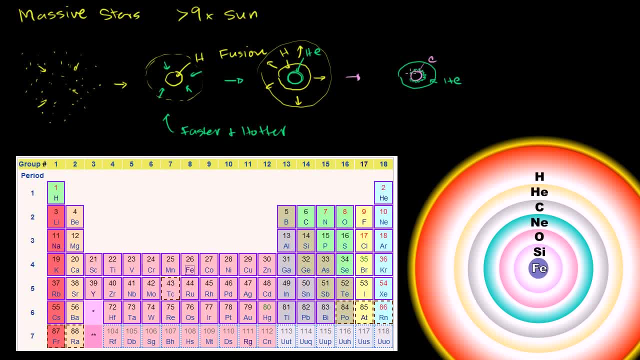 you have a shell of helium fusion, That's helium, not hydrogen, turning into carbon, making that carbon core denser and hotter, And then around that you have hydrogen fusion. Have to be very careful. You have hydrogen fusion And then around that you have the rest of the star. 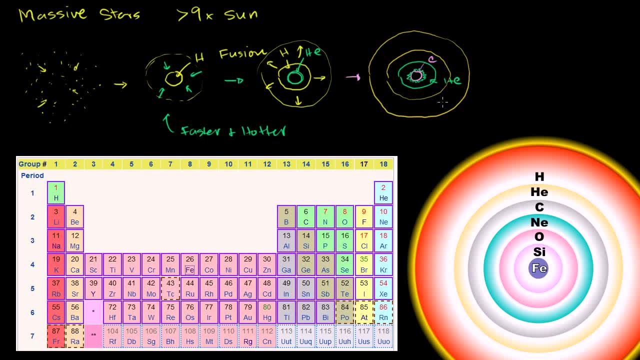 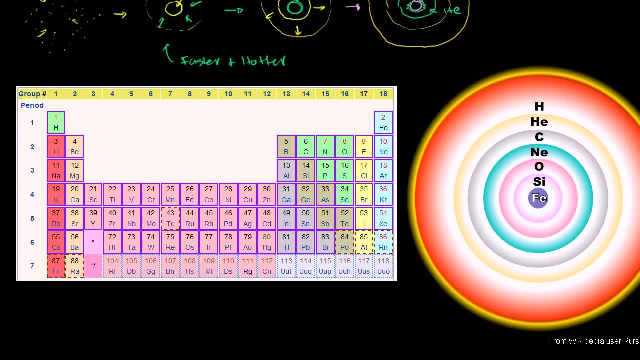 You have the rest of the star, And so this process is going to keep continuing. Eventually, that carbon is going to start fusing And you're going to have heavier and heavier elements form the core, And so this is a depiction off of Wikipedia. 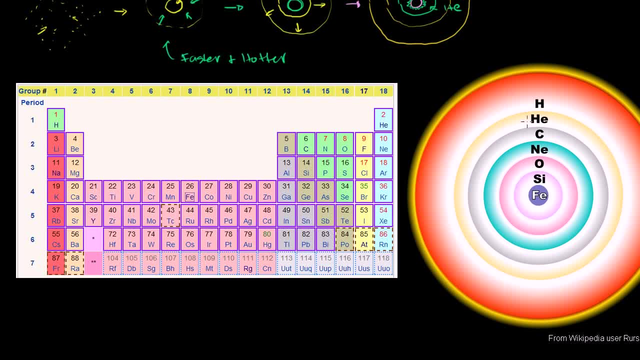 of a fairly mature massive star, And you keep forming these shells of heavier and heavier elements and cores of heavier and heavier elements until eventually you get to iron, And in particular we're talking about iron-56, iron with an atomic mass of 56.. 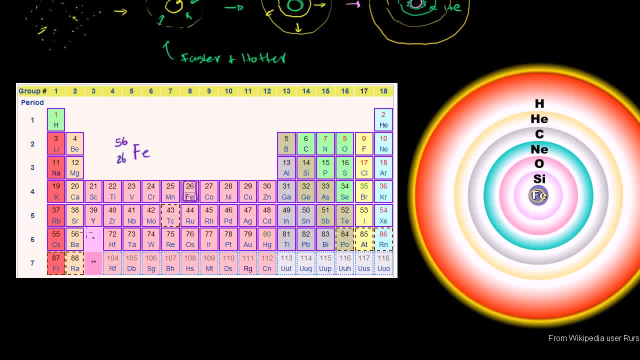 Here on this periodic table, that 26 is its atomic number. It's how many protons it has: 56. is you kind of view it as a count of the protons and neutrons, although it's not exact, But at this point, the reason why you stop here. 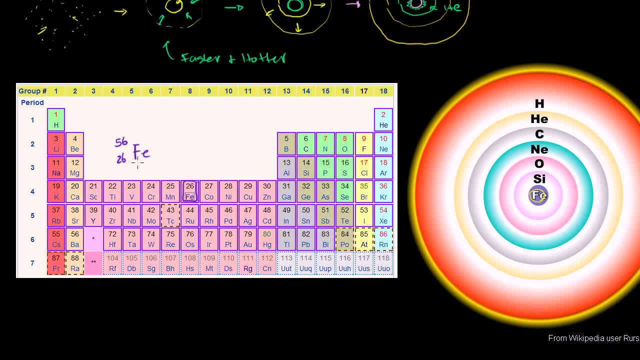 is that you cannot get energy by fusing iron. Fusing iron into heavier elements beyond iron actually requires energy, So it would actually be an endothermic process. So to fuse iron actually won't help support the core. So what I want to do in this? well, just to be very clear, 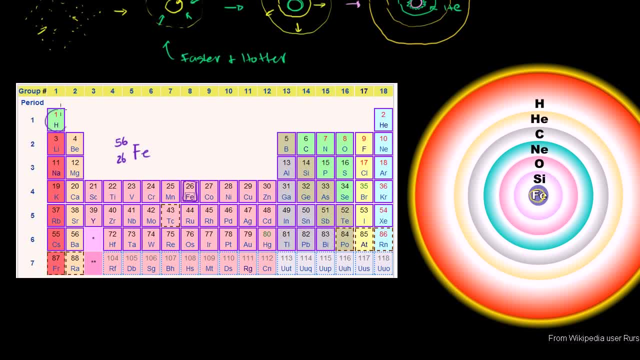 this is how The heavy elements actually formed. We started with hydrogen, Hydrogen fusing into helium, Helium fusing into carbon, And then all of these things in various combinations- and I won't go into all of the details- are fusing heavier and heavier elements. 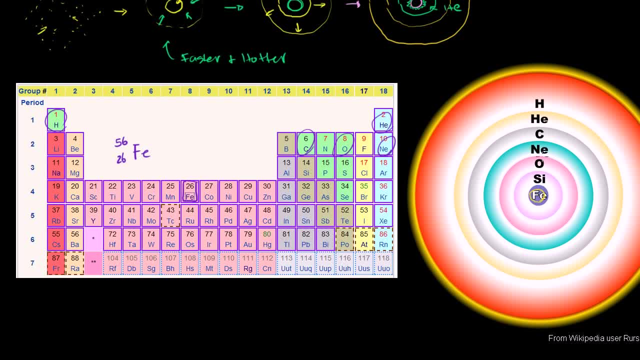 Neon, oxygen and- you see it right over here- silicon, And these aren't the only elements they're forming, but these are kind of the main core elements they're forming. But along the way you have all this other stuff: Lithium, beryllium, boron, all of this other stuff. 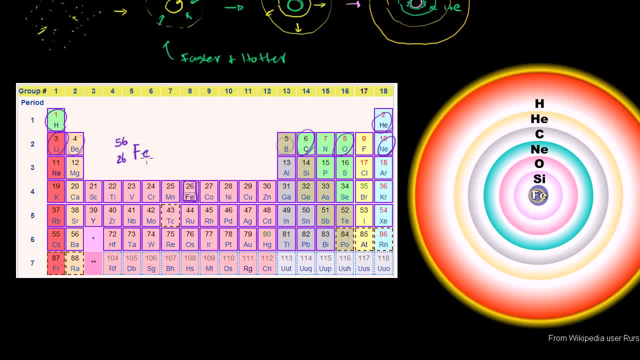 is also forming. So this is how you form elements up to iron-56.. And also, actually, this is actually how you can form up to nickel-56,. just to be exact, There will also be some nickel-56, which has the same mass as iron-56,. 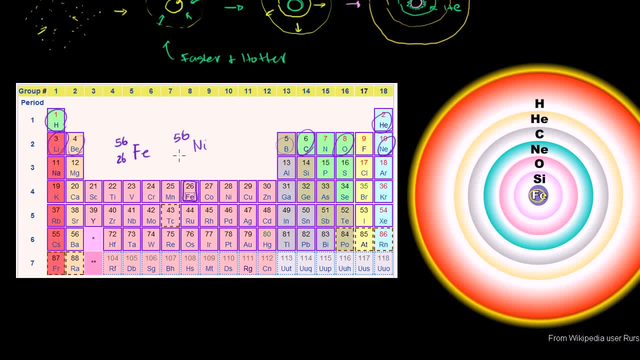 just has two fewer neutrons and two more protons, So it's nickel-56.. Will also form, can also kind of be a nickel-iron core. But that's about how far a star can get, regardless of how massive it is at least. 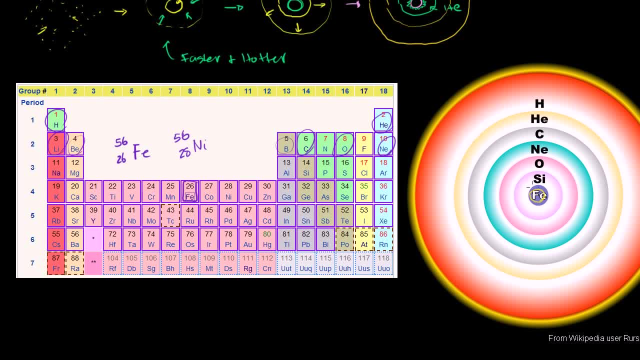 by going through traditional fusion, through the traditional ignition mechanism. What I want to do is leave you there, just so you can think about what might happen next, now that we can't fuse this star anymore And what we're actually going to see is that it will supernova.